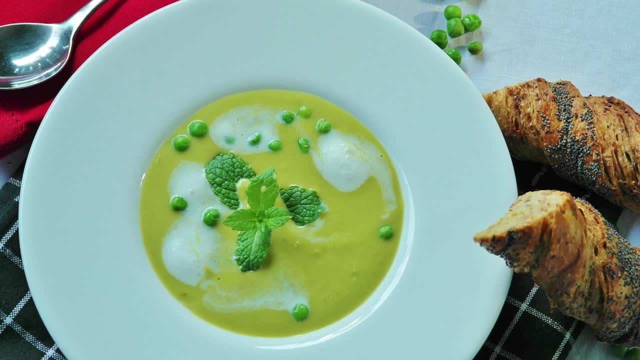 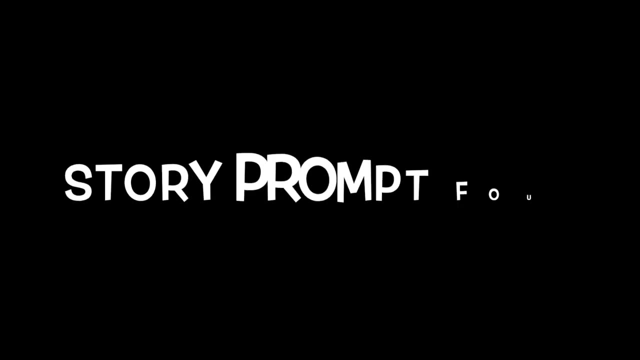 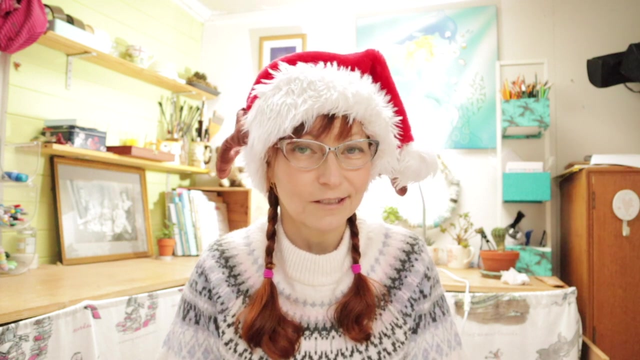 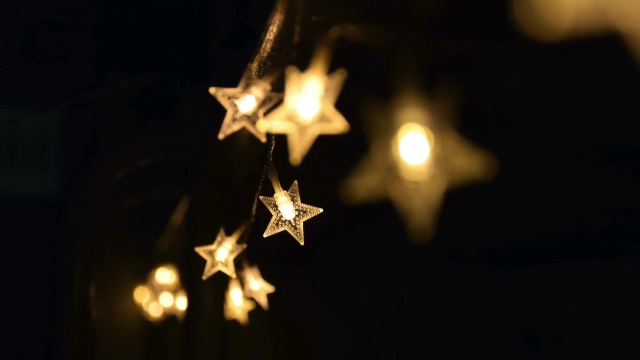 when you crunch into them, or maybe it's the green pea chasing it around the plate with your fork. number four describe Christmas through the eyes of a small child. do they see Santa? what about opening the presents? and what do they like to eat? zoom in on one of those moments to get the best out of a bit of. 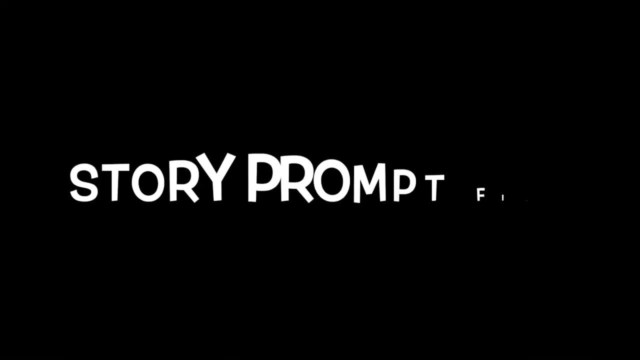 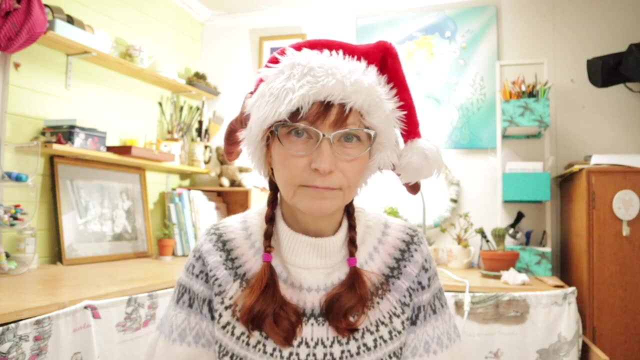 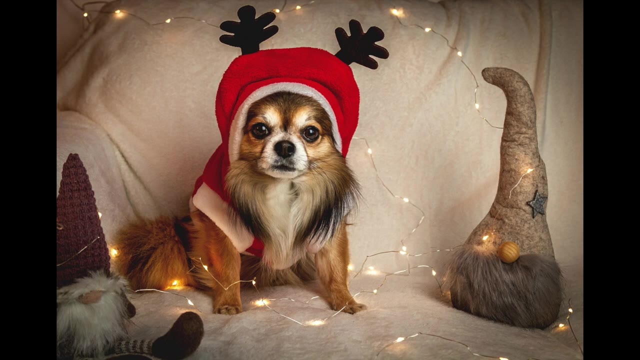 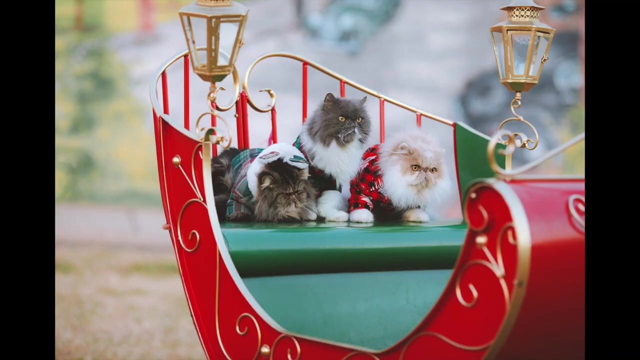 descriptive writing number five: what is Father Christmas doing right now? you know, whatever day it is today in the real world when you are watching this, what do you think he will be doing? crazily wrapping presents, getting himself sleigh-ready- maybe it's Christmas Eve- or having a long nap in. 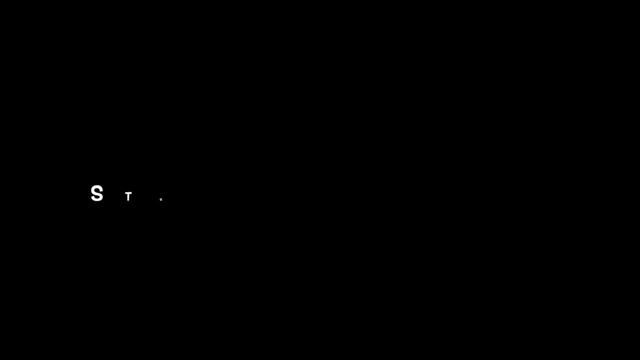 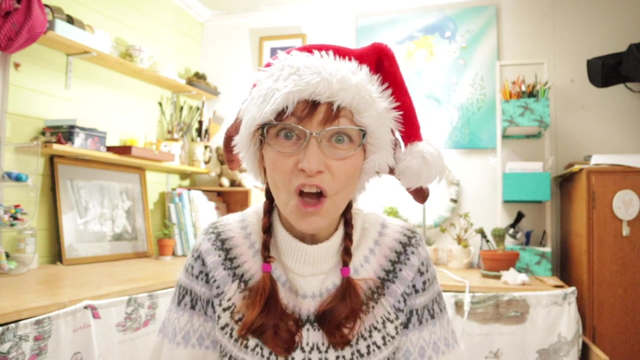 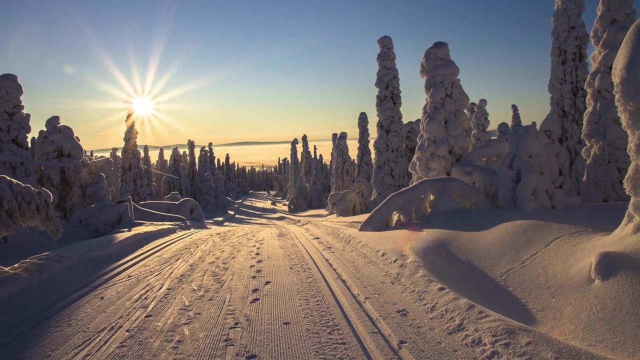 the aftermath of the big day number six, mum and dad wake up on Christmas morning and there's a note from the children saying they've gone back to Lapland with Father Christmas. Whose viewpoint are you going to write your story from? The parents or the kids? 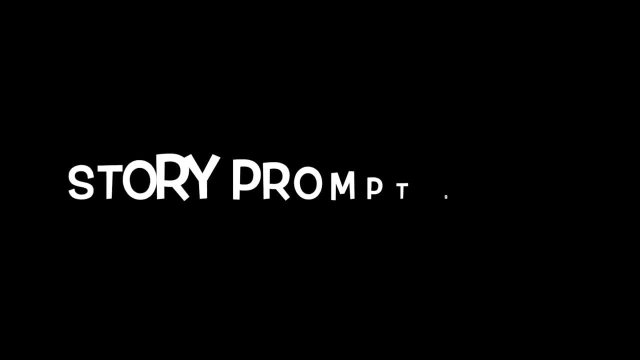 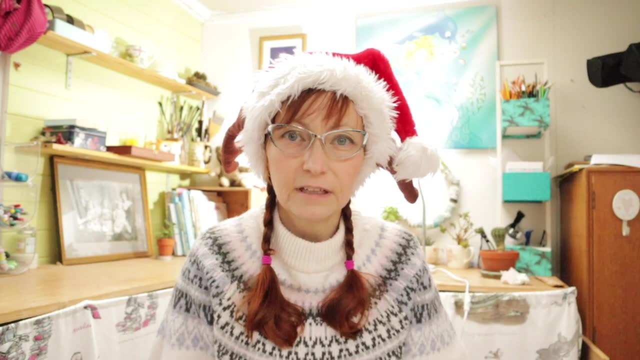 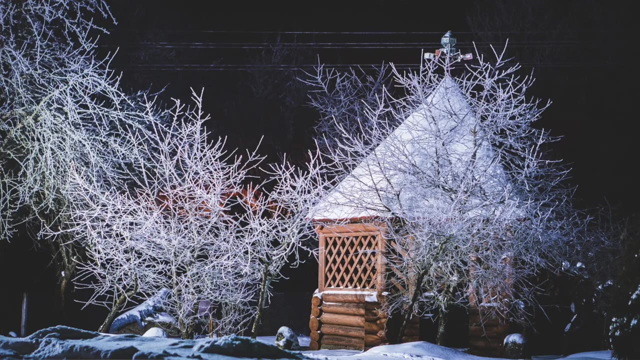 And what are they doing? Number seven: It's Christmas Eve and you can't sleep. Eventually, you get up out of bed and look out of the window. What do you see? This is a great idea. Is it snow Or is it a burglar? 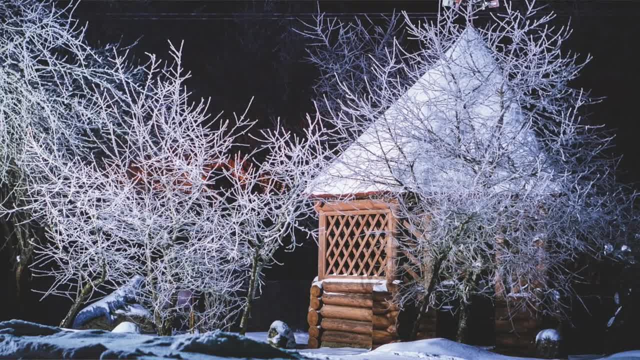 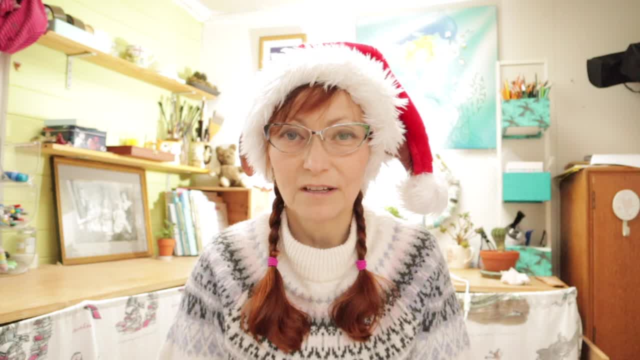 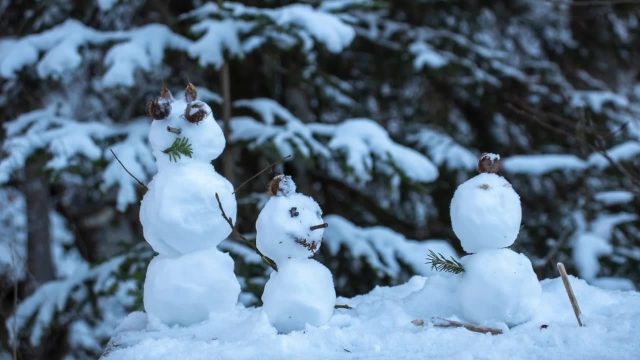 Or is it a lost dog playing with a snowman? Choose the first line of a famous Christmas song and use it as the first line of your story. Like last Christmas, I gave you my heart, but the very next day you gave it away. 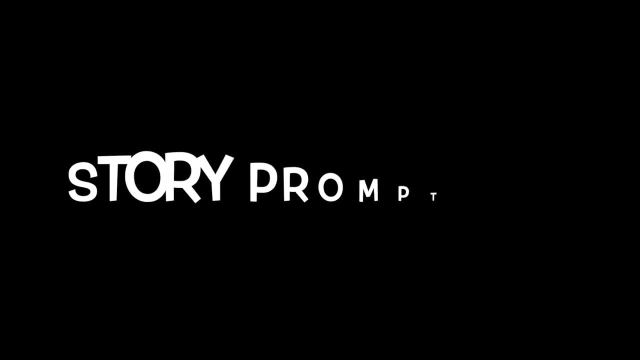 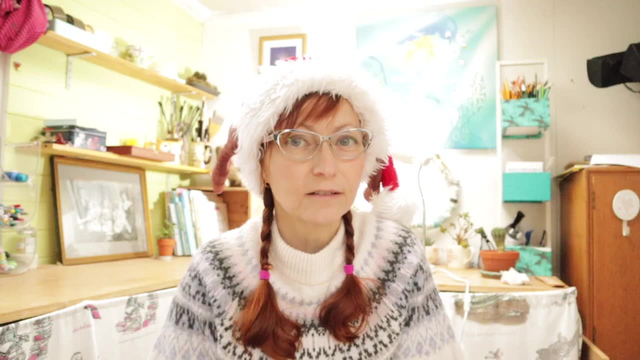 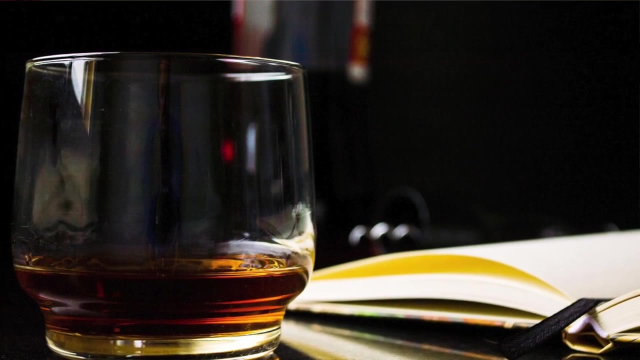 Where are you going to go with that Number nine? You're in an old pub on Christmas Eve. as the snow starts In comes an old man wearing a hooded cloak. He sits down next to you with a mug of ale and starts to tell you his night before Christmas story.